For example, if you have a plant that needs full sun, you would want to choose a plant that has a similar or complementing shade or sun and water requirements. For example, if you have a plant that needs full sun, you would want to choose a plant that has a similar or complementing shade or sun and water requirements. For example, if you have a plant that needs full sun, you would want to choose a plant that has a similar or complementing shade or sun and water requirements. For example, if you have a plant that needs full sun, you would want to choose a plant that has a similar or complementing shade or sun and water requirements. 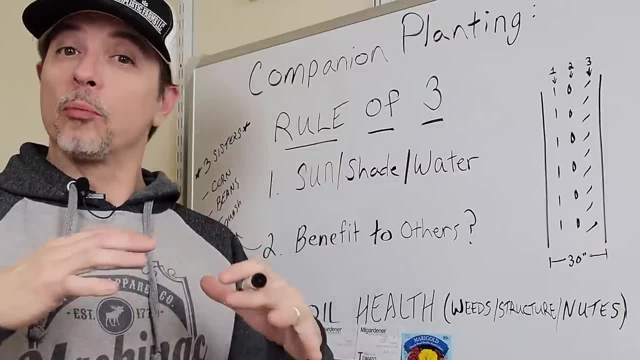 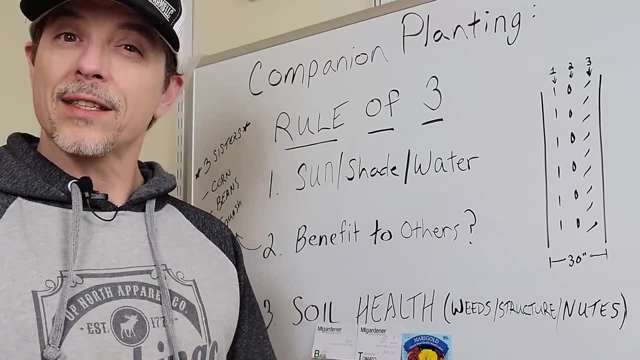 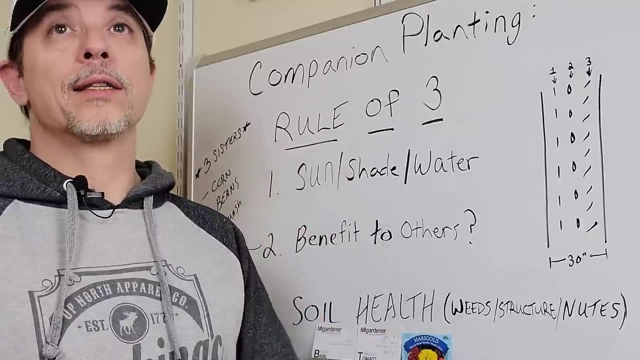 soils. other plants will have shallow roots that can help prevent erosion. some plants will attract beneficial insects that'll kind of control pests, while other plants you can actually repel pests. another great method is I'll use plants that will create shade for more delicate plants. I use that one a lot, so 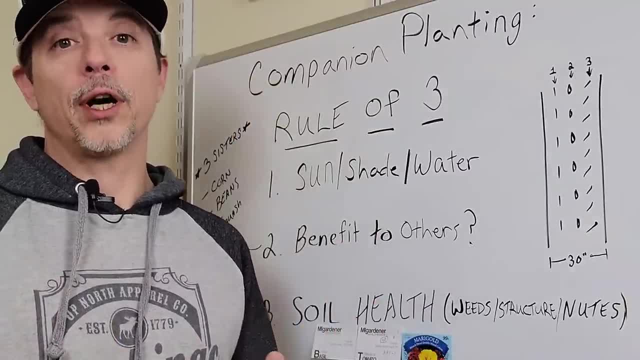 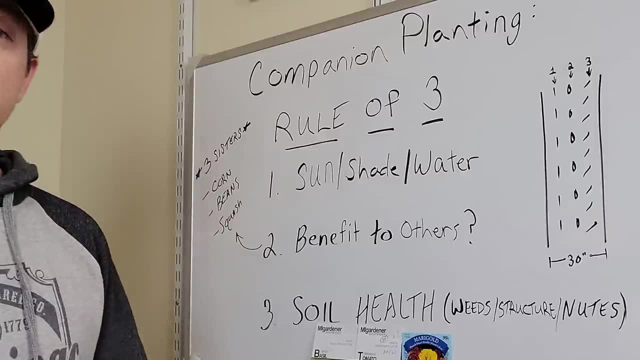 by pairing plants that complement each other, you create a healthier, more productive garden. I think one of the very best examples of this is actually the three sisters method the Native Americans used to use. they would plant corn beans and squash. the corn would act as a trellis for the pole beans to grow. 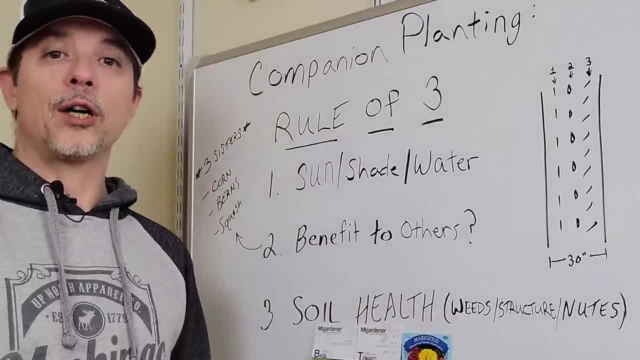 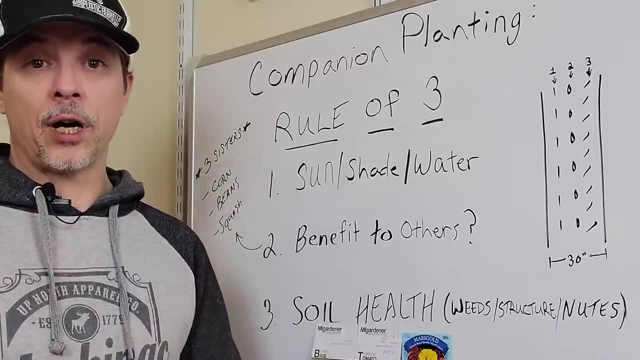 up the beans would provide nitrogen for the corn and the squash, and the squash could grow down low and act as a weed suppressant. it worked phenomenal and they all benefited off each other all right now the third factor I like to look at is: does it improve the soil? 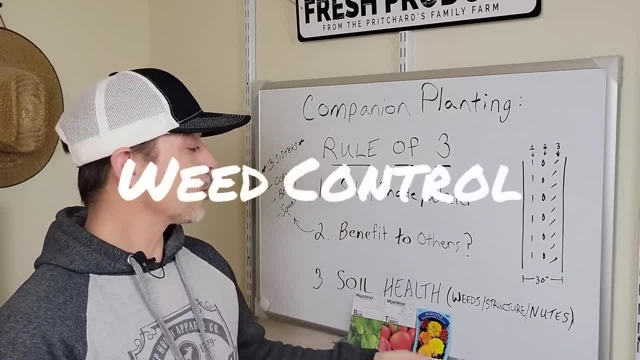 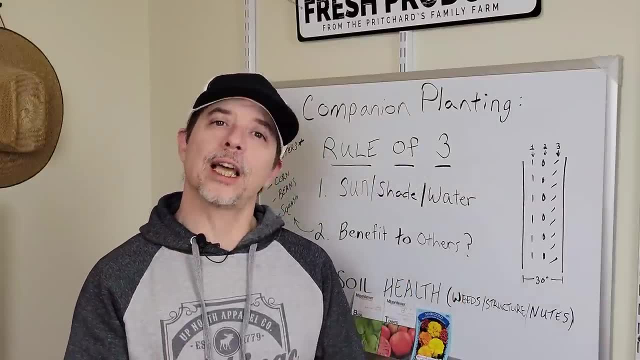 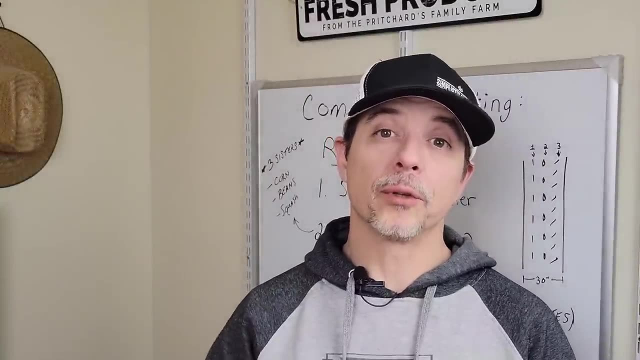 I try to think of it in terms of weed control, soil structure and nutrients. now some plants, such as your legumes, your beans and your peas- they actually have nitrogen fixing bacteria on their roots, so they can definitely enrich your soil with nitrogen. other plants have deep tap roots which can help break up compacted 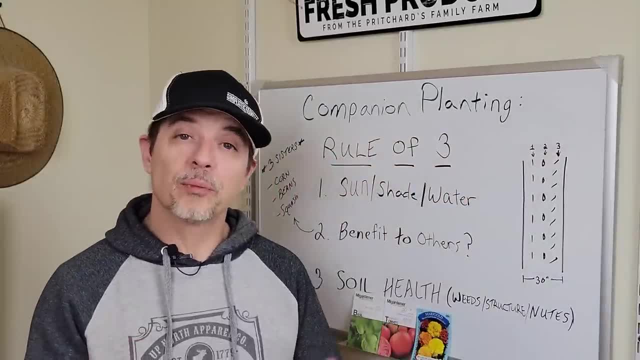 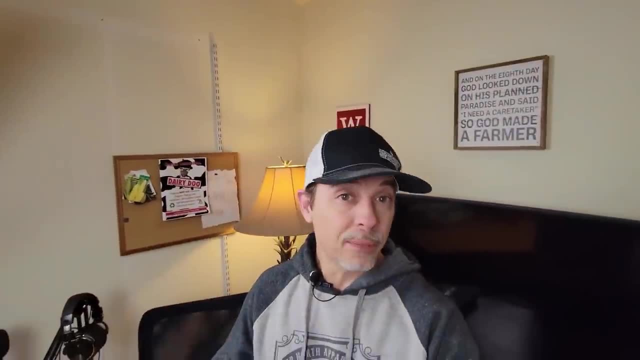 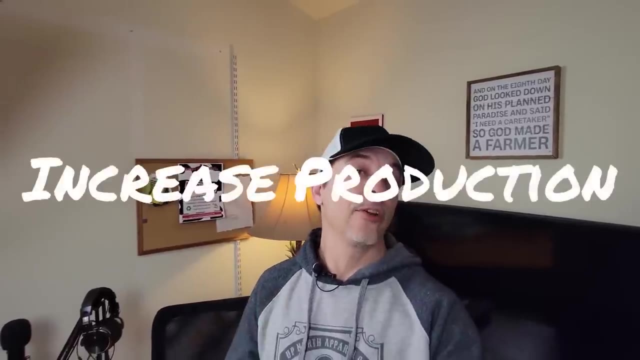 soil. improve your drainage now. by choosing plants that improve the soil, you're creating a much healthier environment for all your plants in the garden. now, of course, companion planting can have many additional benefits, can definitely maximize space by growing vertically. you can really increase production by utilizing all the space in your garden beds, and it'll even make it look a 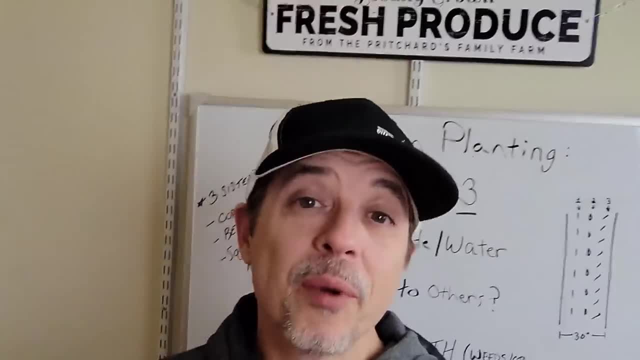 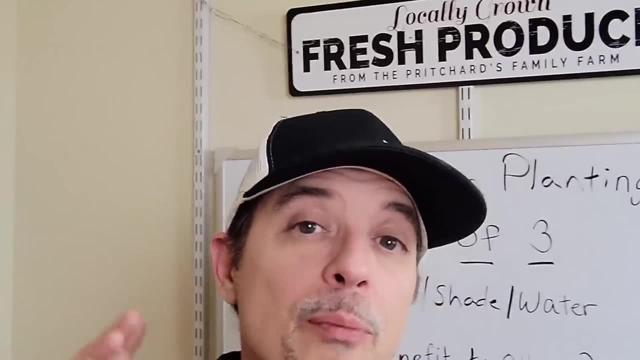 little more beautiful with all the different colors and textures. now I'm going to give you a list of five groupings of companion plants that we use out in our garden every year and you can use in yours this year to make it a little more simple. but before I do, do me a favor if you're getting some value out.